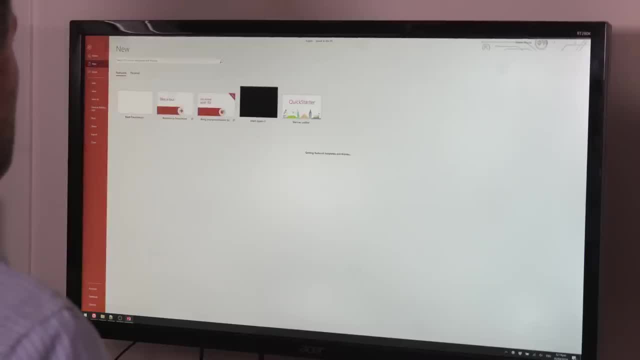 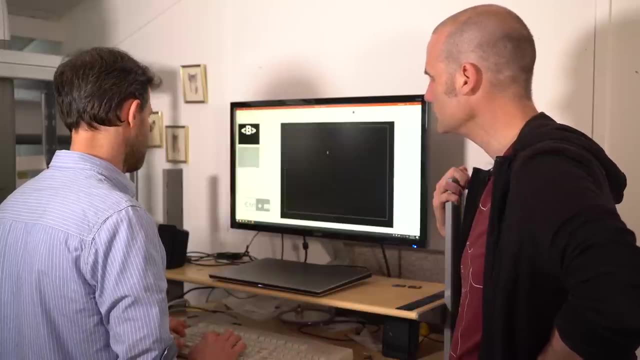 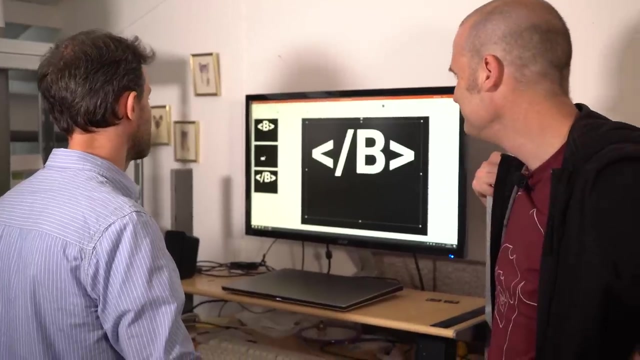 and then we'll start with a new one and we're going to call this one presentation B. Okay, All right, let's do a couple of new slides and then close that presentation. All right, now this slide, the middle slide of presentation B, I'm going to insert. 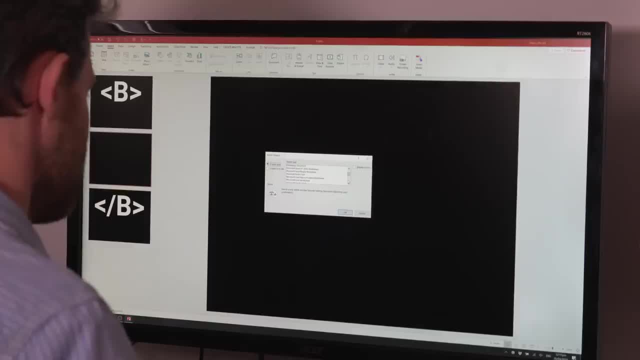 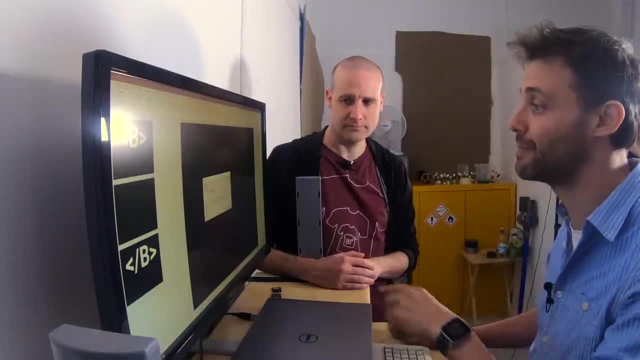 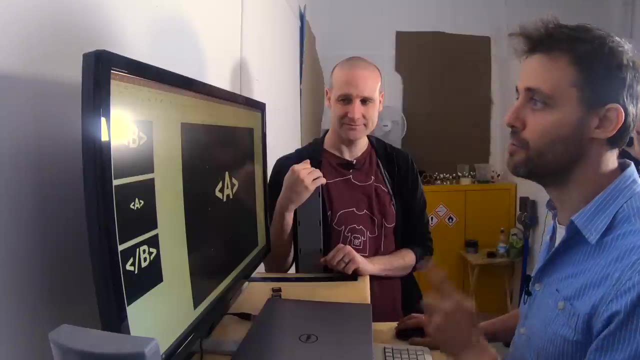 an object, a PowerPoint presentation. But what presentation? We're going to embed PowerPoint A and it's going to be a link. Okay, so there we go. Oh, so you've linked to the first. Yeah, That's so good. Then what you've got to do is you've got to go into animations, add animation and this: 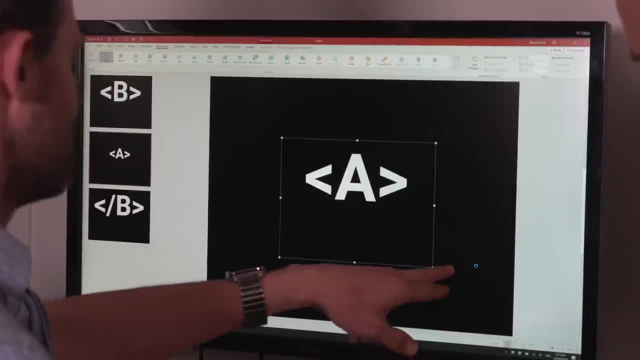 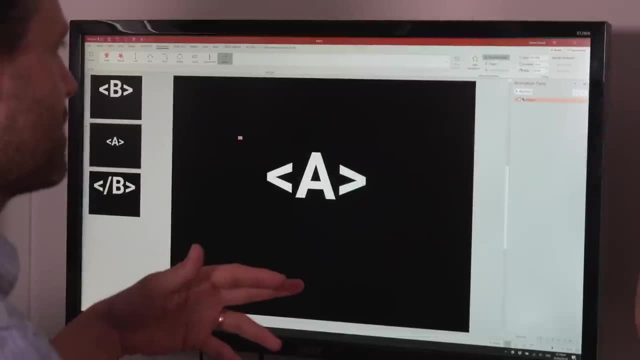 presentation needs to automatically start on the click. So we're just going to do show, Okay, so we're going to show the presentation and that's going to happen. let's do it not on the top but on the bottom, Not on click, but start with previous Okay. so now let's start the presentation again. 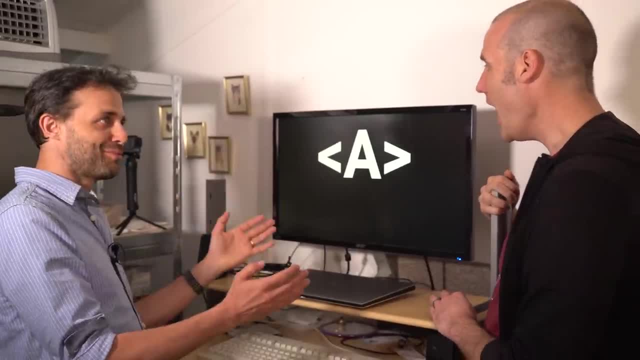 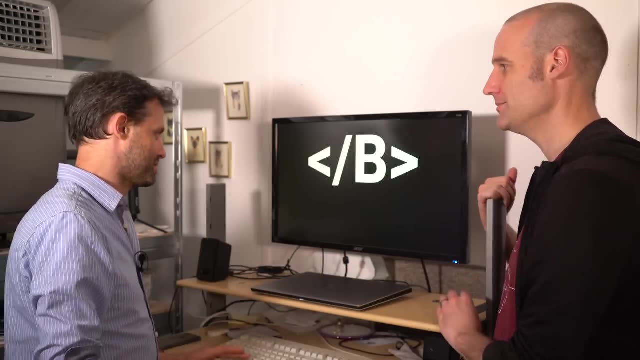 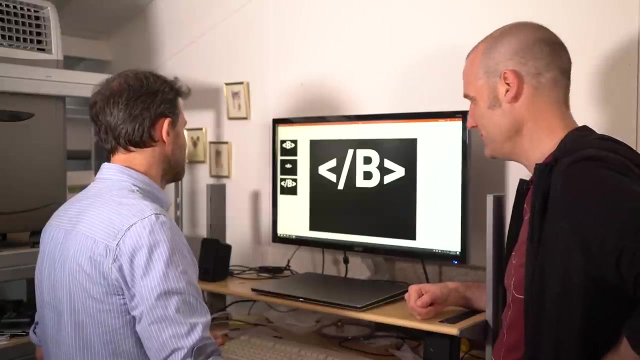 Presentation B. Okay, now we're in presentation A and you can go through presentation A and then you drop out again and then you finish presentation B. Okay, it's fairly straightforward and any changes that I make to presentation A automatically propagate to here. But let's go into presentation A now and insert presentation B into presentation B. 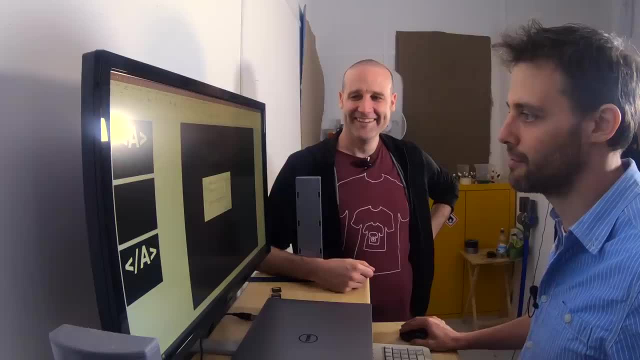 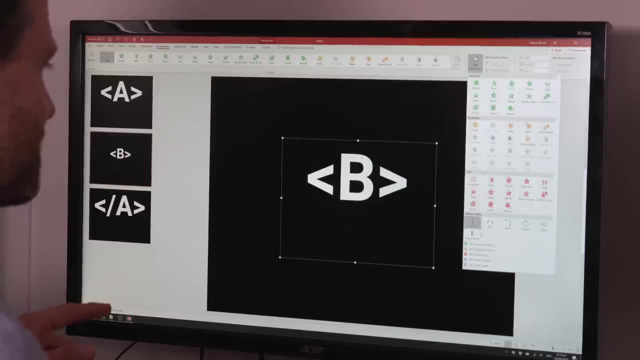 Okay, Oh, this is brilliant. Okay. insert object: create from file browse. Presentation B is now going into presentation A. Start it in the click sequence. This is way easier to use than Keynote. You couldn't do this in Keynote. 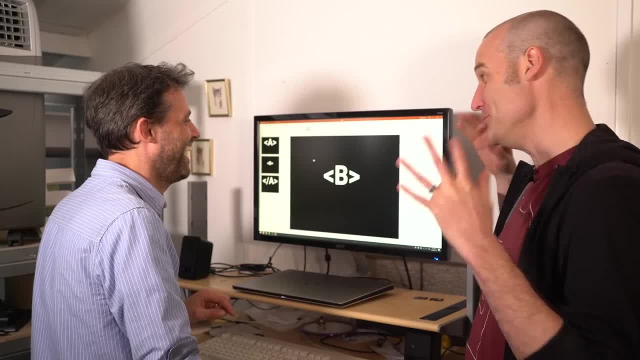 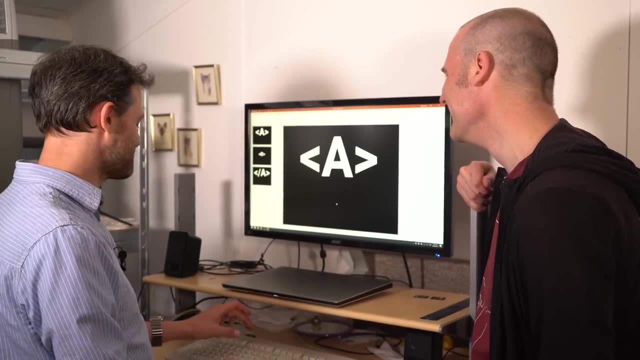 So true, so true, The price you pay for usability. So A presentation A is embedded in presentation B. presentation B is embedded in presentation A. Let's start presentation A now. Okay, so look, we're going through Into B. Yeah, Into B. 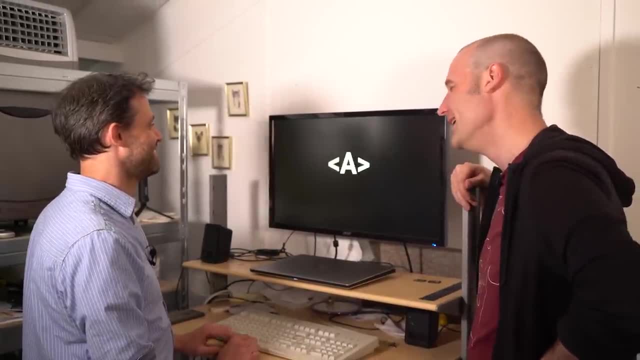 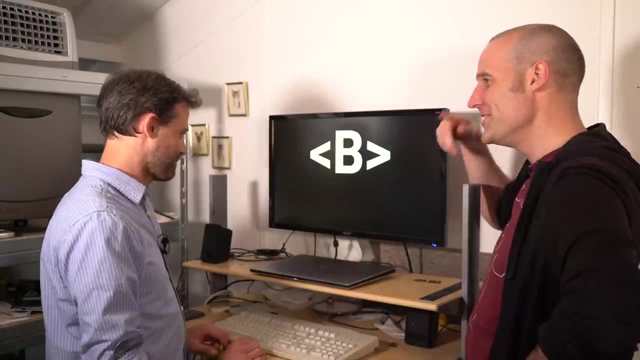 But then the second slide of B is A- A, And then the second slide of A is B. Yeah, Brilliant. So now look, I cannot get to the end of a PowerPoint presentation. It doesn't matter how hard I try. You're a little infinite loop there. 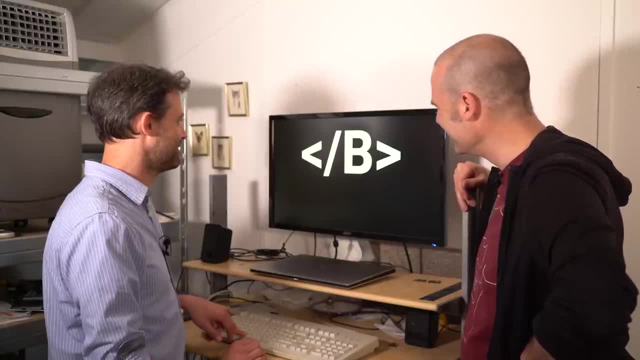 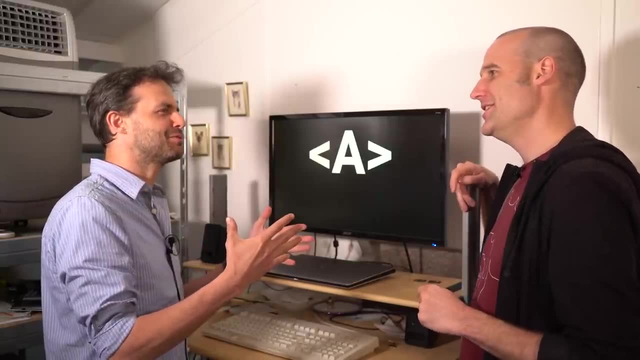 Yeah, yeah, Look, just if I hold it down, What happens weirdly is sometimes it will. it's like it's a race error or something like that. What do you call it? Basically, you're skipping over it before it has a chance to load. 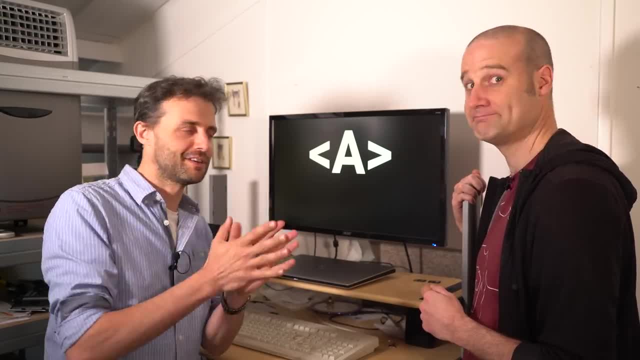 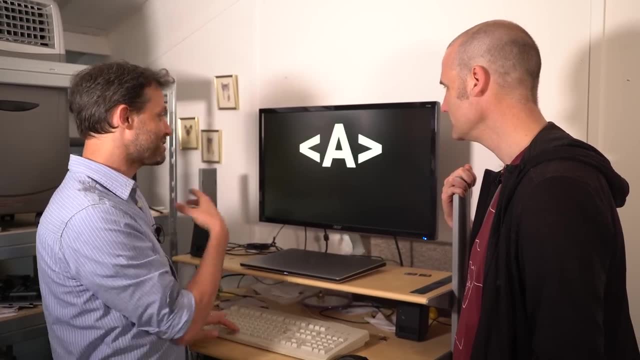 Yeah, yeah, Yeah, no, yeah. someone said so. I did this in an evening of unnecessary duty, Which is a live thing, and someone came up to me and said: it looks like a race condition. Like you know, one thing is coming ahead and yet it still doesn't. let you get out. 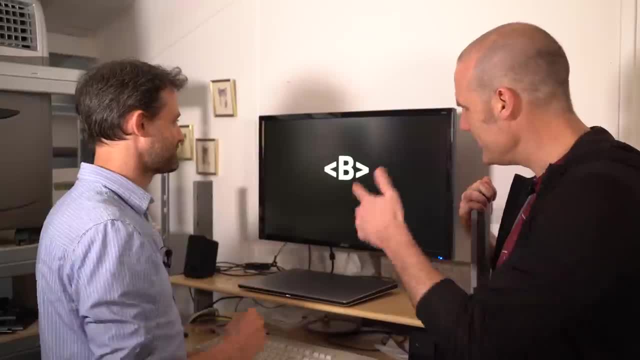 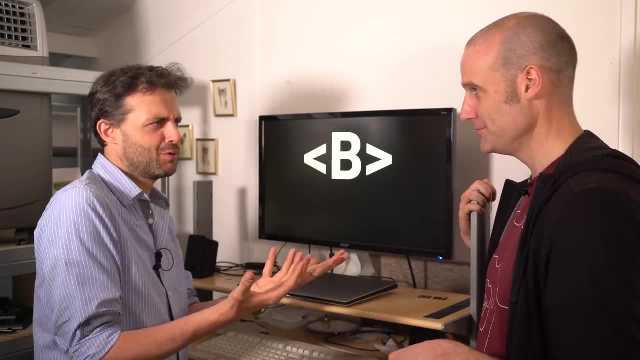 Even if you race ahead, it never hits. how deep are we now? Yeah, it is the fun part. If you want to escape out of a presentation, what do you do? Hit escape, Hit escape. That just came out of A presentation. 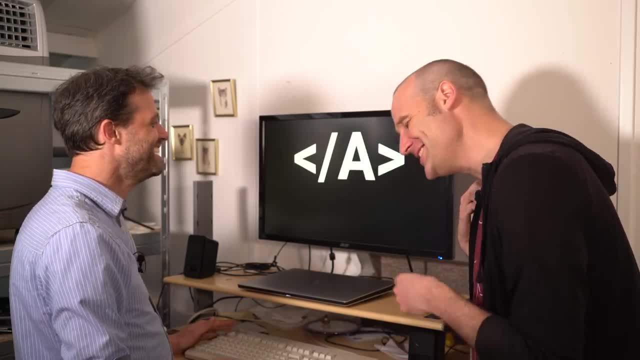 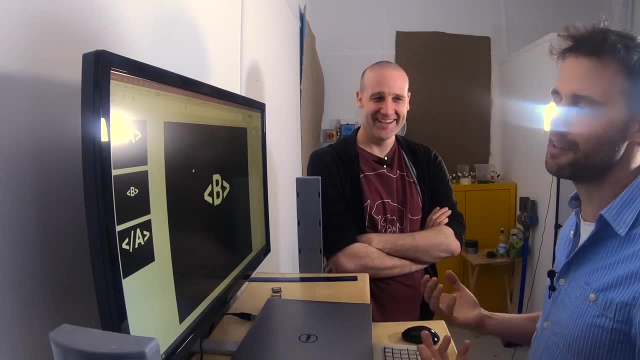 Yeah, So you've got to hit that as many times, so we're going all the way back up the level. Okay, okay, This could take a second. Yeah, Oh, no, it doesn't Okay. So there you go. so that was the fun thing that I showed you. 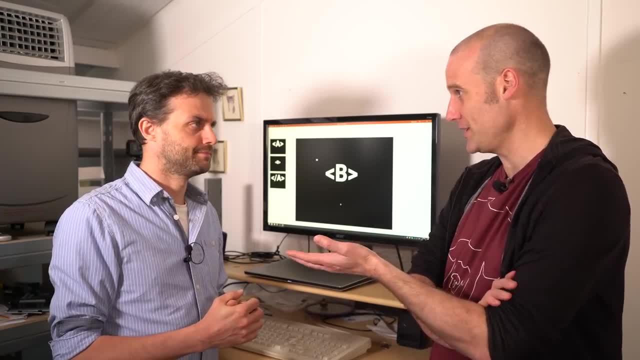 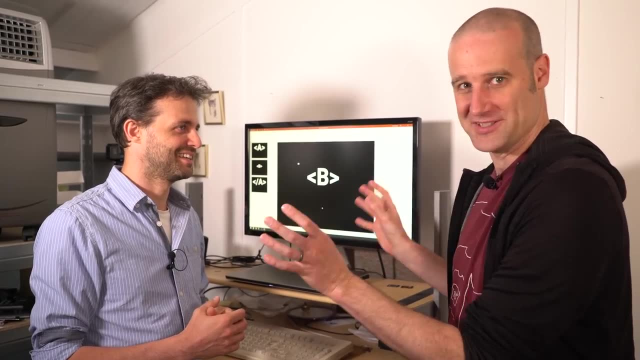 So, like Steve said, we did this at an evening of unnecessary detail and the audience. we had a good old chat about how much memory and all that And then I said: can you embed more than one version of the presentation in the presentation? 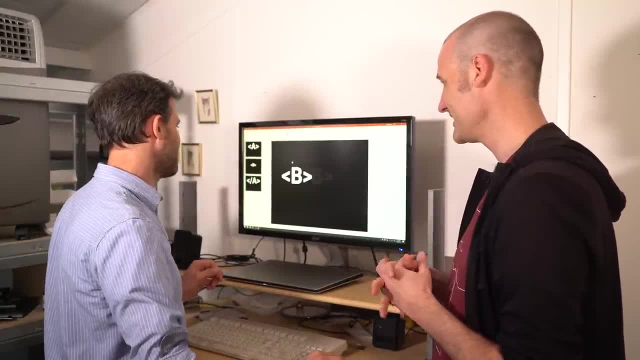 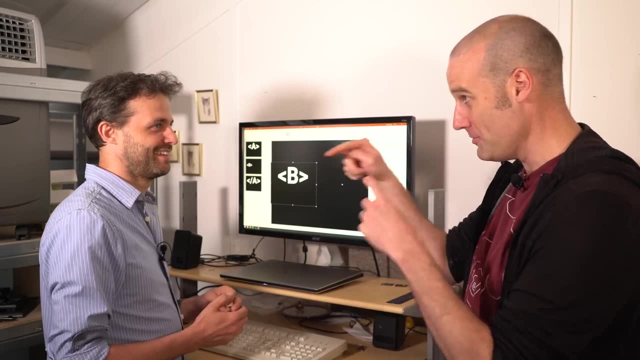 Yeah, so like could I do presentation B and another presentation B. here I was thinking you could generate fractals, because if you even put it into itself and multiple copies, you could start to get these fractal structures. And this is what you think you've done. 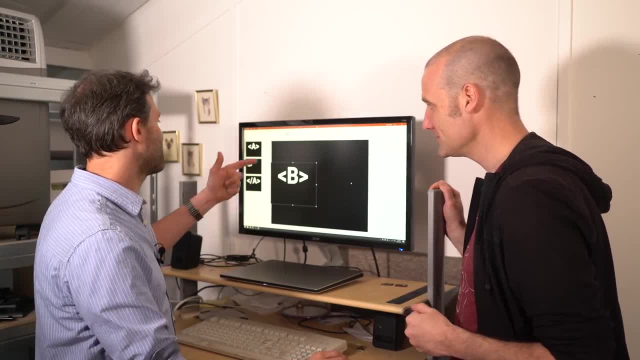 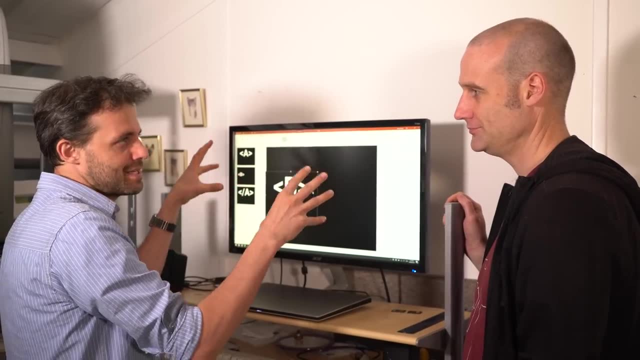 Yeah, so unfortunately, whenever you start playing the presentation, it goes full screen. So even if you had two, it would just full screen. one of them Full screen, one of them right. So you're never going to get this kind of shrinking in like that. 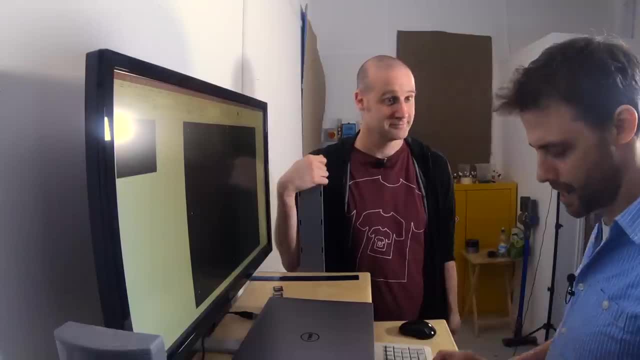 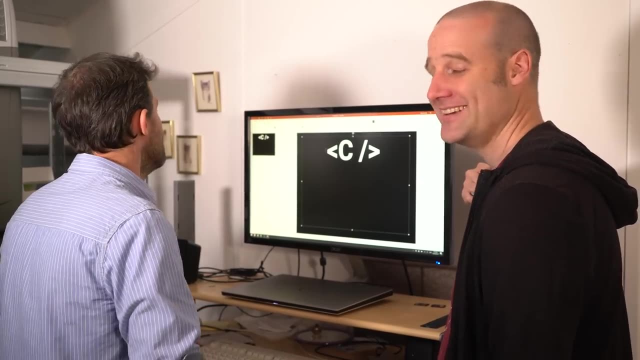 But this is what I found out. Okay, presentation C now only has one slide, So let's close that. That's how you self-close. Oh good, It's his favourite programming language. It is, I'm joking, It's not really. 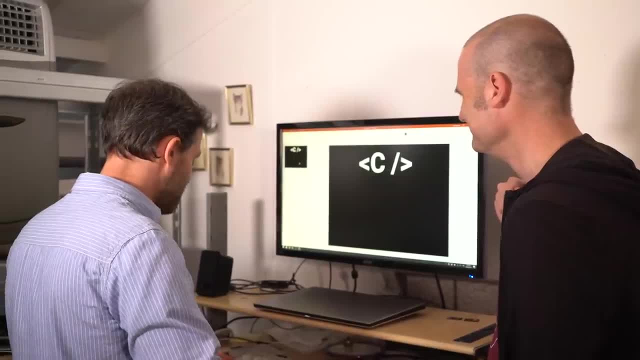 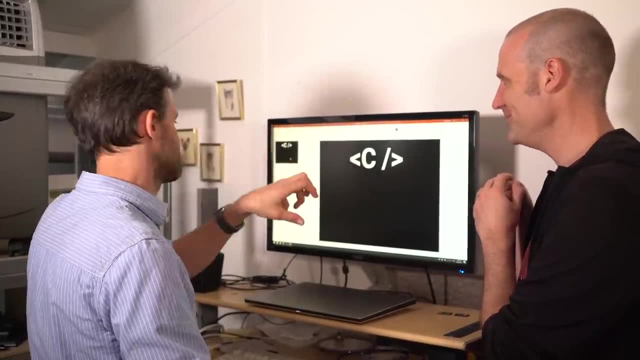 It's CSS. Okay, so now we're going to copy a slide this time, So we're not embedding PowerPoint presentations within each other. we're embedding slides within other slides, So we're going to take this slide. we're copying this slide. 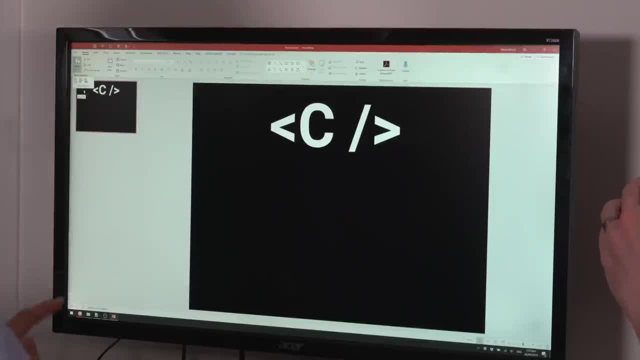 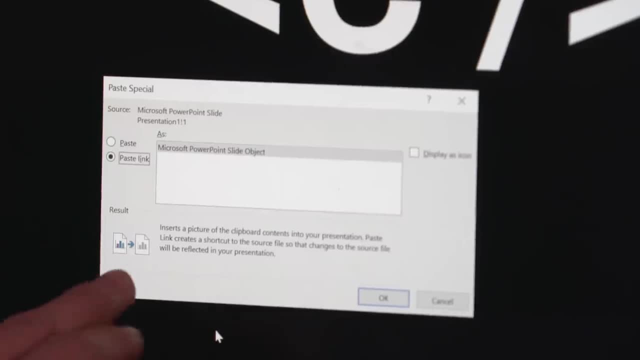 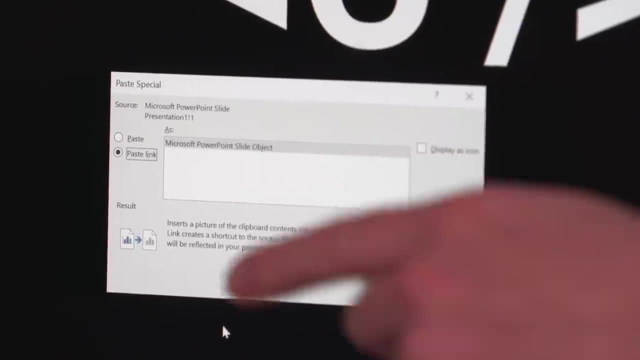 and then we're pasting the slide into itself. But we're doing paste special, Not just any kind of paste, Paste link, And what that does is it inserts a picture of the clipboard contents into your presentation, but it's linked Right. so you're posting a link to the slide into the slide. 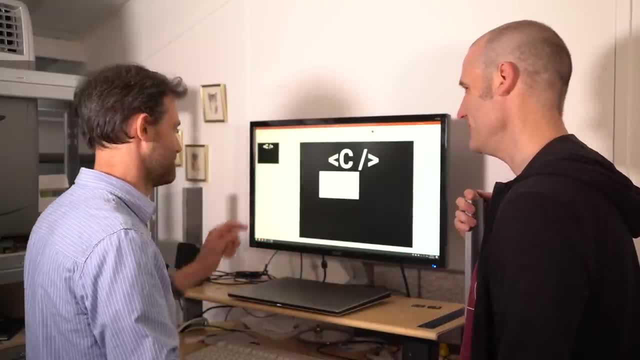 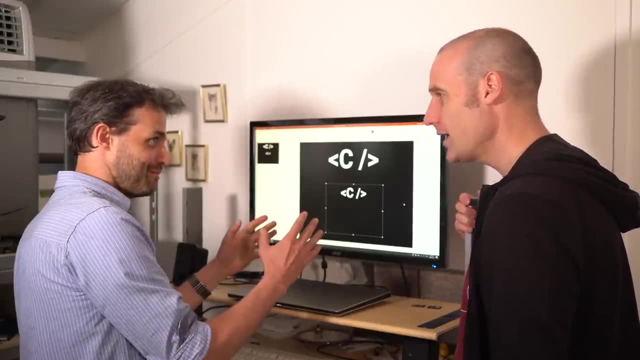 Yeah, as a picture. As a picture, But the picture will update When the slide updates. So there it is. So good, Pop that down there. Okay, So now we're going to save the presentation. Okay, that's good. 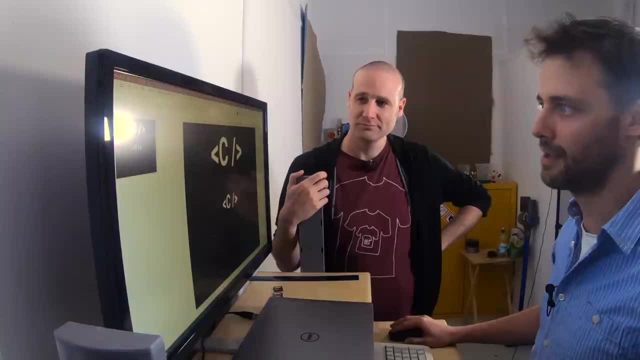 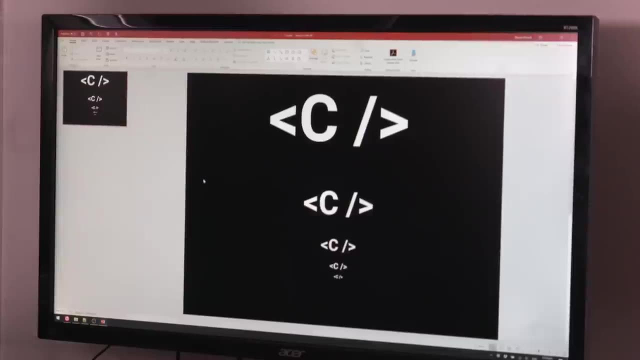 Always save. So just control S, of course. And there's another little one. All right, save it again, Save it again And again and again. There you go, There you go. That is brilliant, So this is the basis for doing something like this. 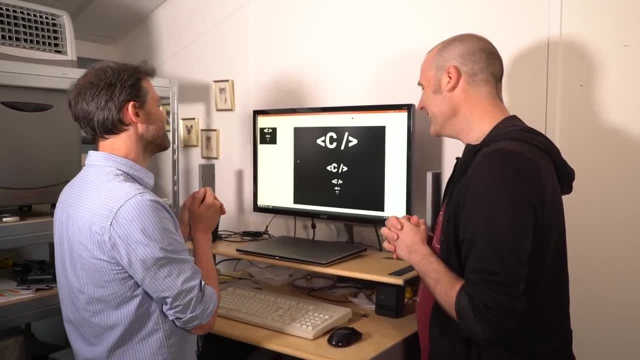 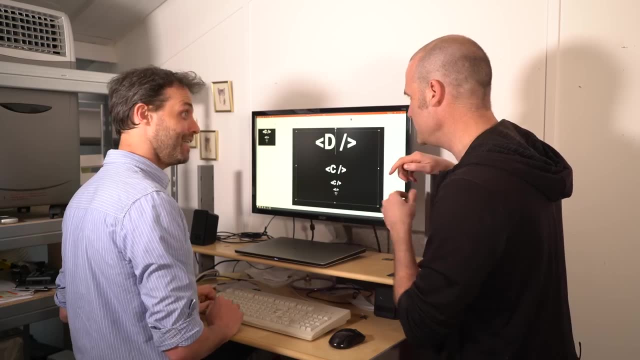 For doing some interesting things, And can I show you some of the stuff that I've come up with? Yeah, like if you change the top one now, will it propagate down? I don't know. D Yeah, yeah, yeah. 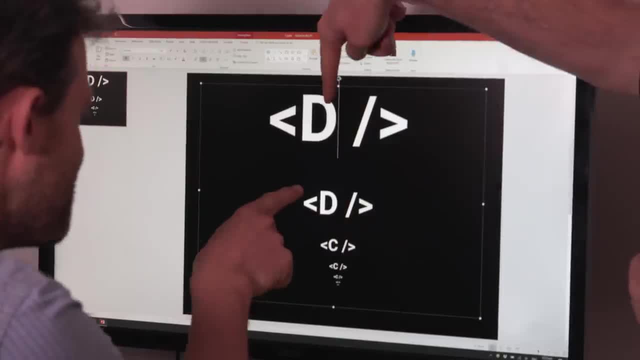 Okay, save, Oh, but it's done there. Put it back to C. It's done there, but I think No, no, Oh, yeah, yeah, Okay, put it back to C, Save, And that D is now just going to. 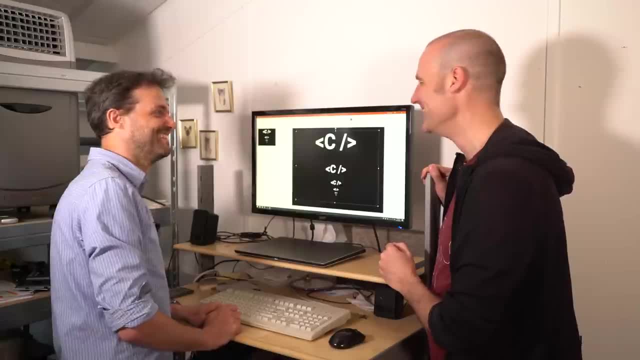 The D is just going to work its way down, Do the thing. Oh, that's so nice, But all that time we've been saving, it's been getting more and more. The Cs are still racing ahead and that D is now chasing it. 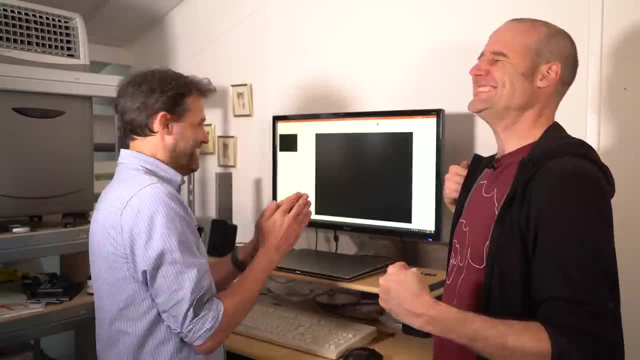 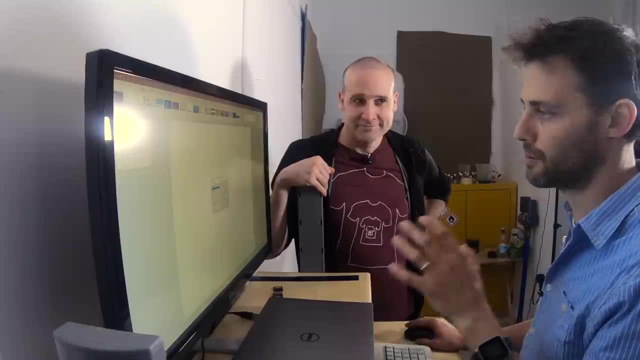 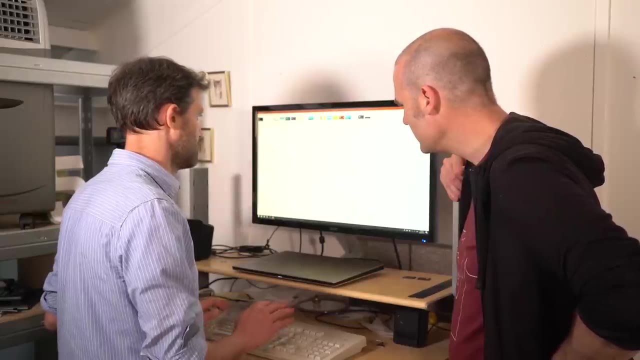 So we're now going to see if we can make our first fractal, Come on, Okay, Let's change the background to white. The first thing I'm going to do is actually make the slide a custom size. I'm going to make it 30 by 30.. 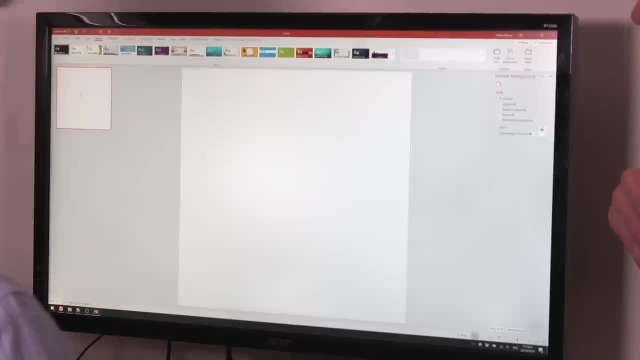 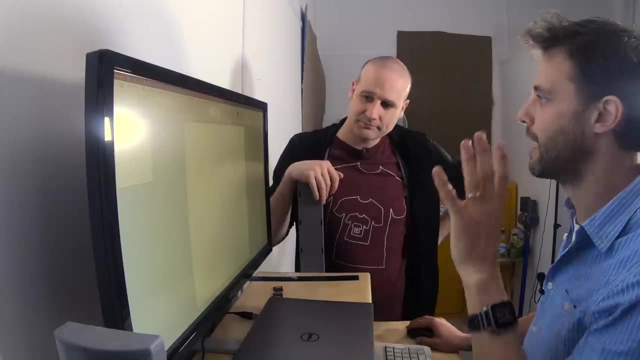 And now it's a perfect square. Okay, so now we're going to take a copy and then paste it in Paste special link. So now I want this to be a third of the full width, In other words, 10.. 10. 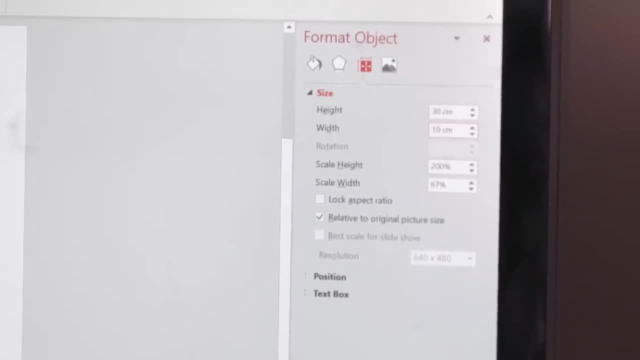 So there we go, Got that now Nice, And now I want another one down here. You might think I can just copy and paste this. I can't. I have to do it all again, which is a weird quirk of the way this works. 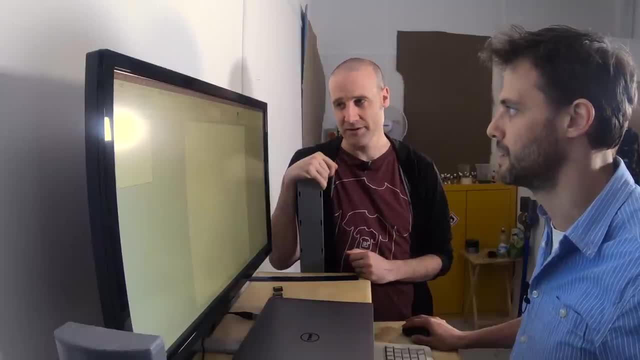 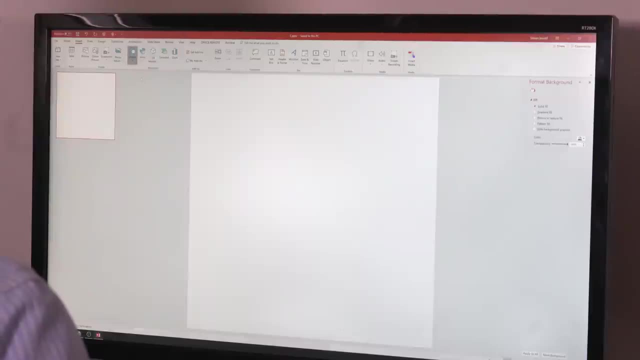 Okay, so Paste it in again. Put it back in the corner. Yeah, stick it in the corner there. And then we need to insert a shape, Just a square. I'll do that And I'm going to make that also 30 high and 10 wide. 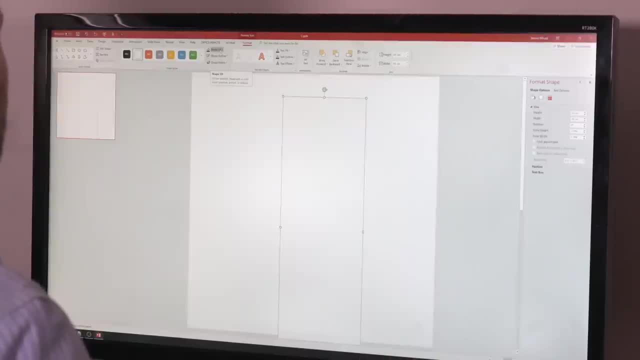 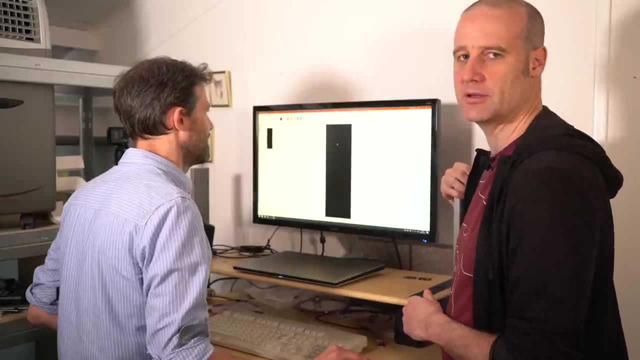 Okay, so that's the middle third. Yeah, Shape fill is black. No shape outline, because that's going to cause us problems anyway. Why would anyone do it differently? Who has ever had a shape outline? Actually, I'm just going to center it on the page, because then I know it's everything. 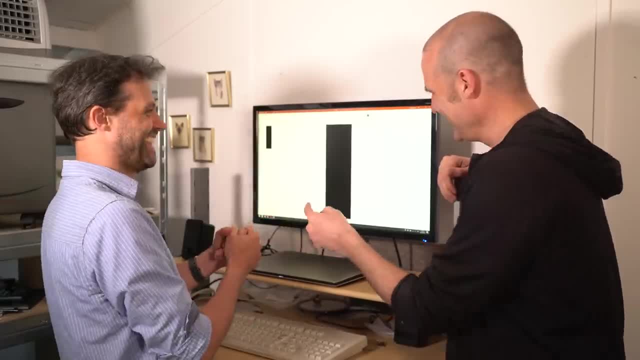 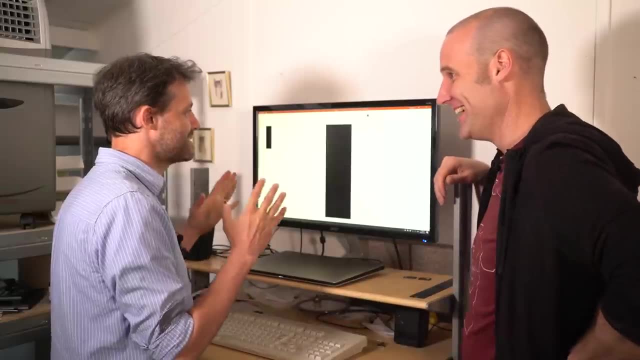 Okay, There we go. So to recap, The whole slide stretched. Yeah, A new black shape? Yeah, The whole slide stretched. Yes, Any guesses as to what this might become? This is feeling very Cantor-y. It's a Cantor set. 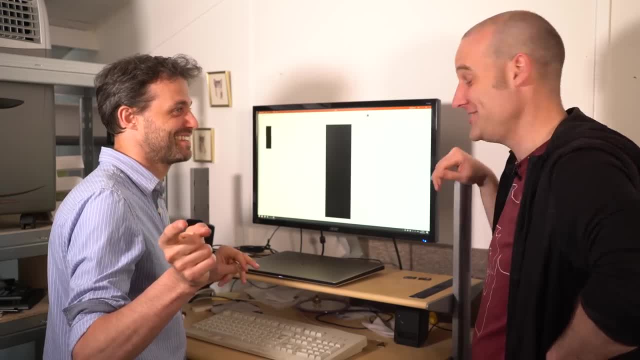 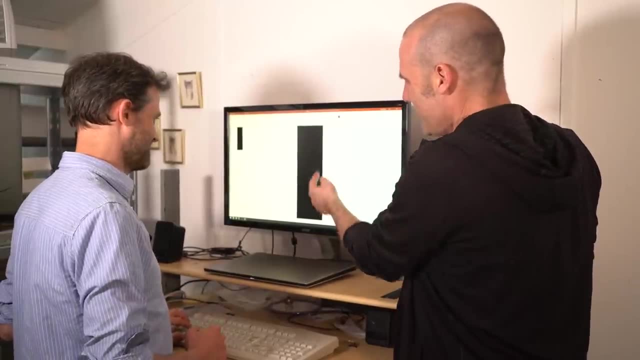 So do you want to tell people how the Cantor set works? Well, you start with a thing and you lop out the middle third. Yeah, And then whatever's left, lop out the middle third. So when you save, currently you've removed the middle third by making it black. 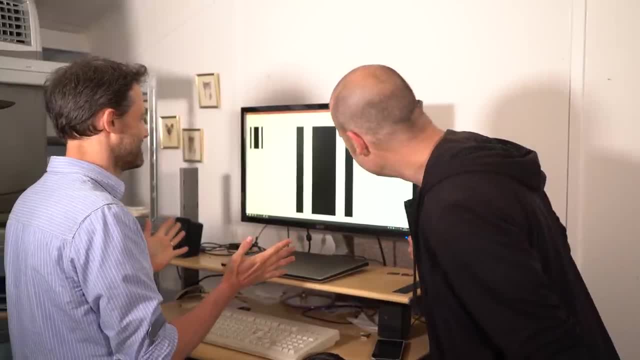 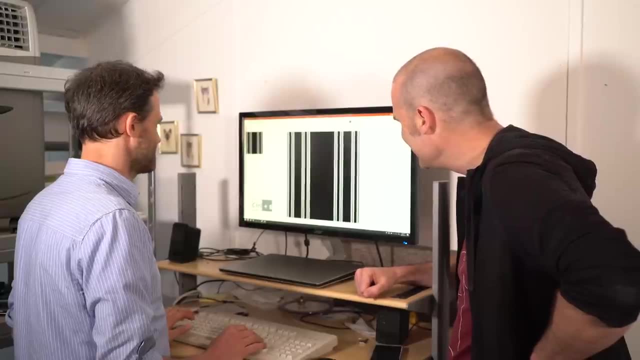 So save Bang. Oh, that's so good. It's taken a third out of. If you save again, do we do it? There you go, Oh, keep going, Don't stop. That's amazing. And that is the Cantor set. 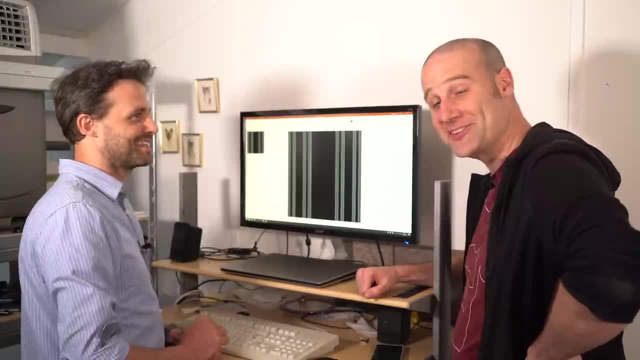 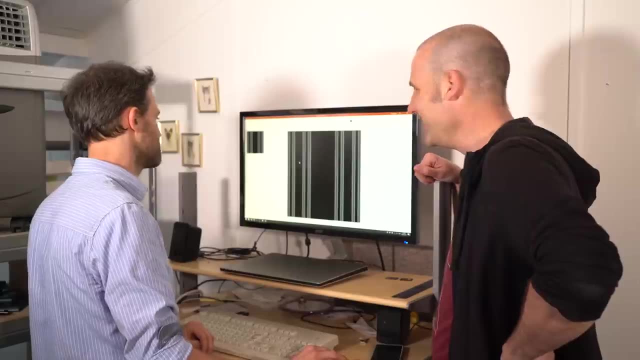 Classic, A famously underwhelming fractal. It's amazing that you built it in PowerPoint, though. That's very cool, Which is why? because it's underwhelming. I've got a slightly more interesting one, So for this one, let's get rid of all of that. 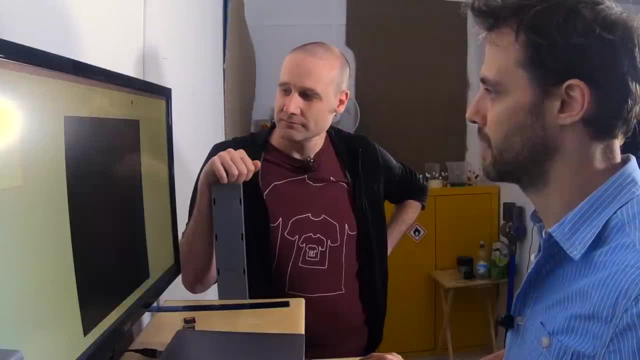 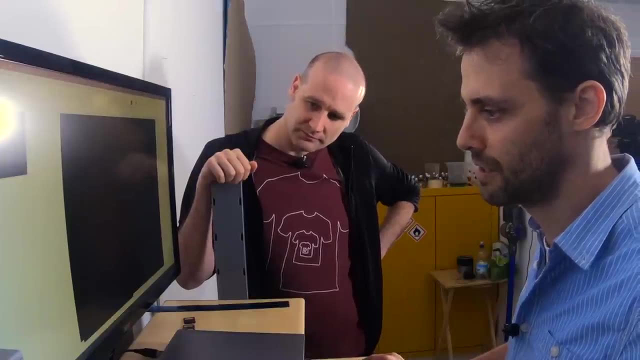 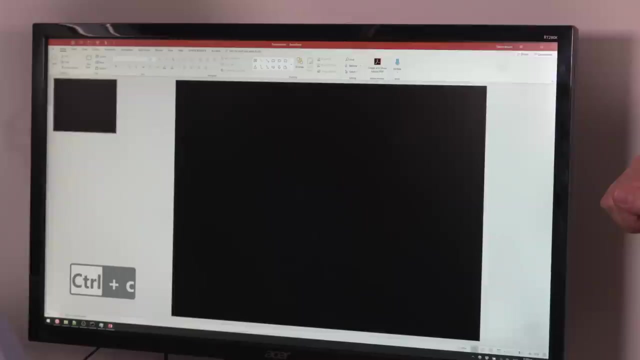 In fact, let's make the background black. Okay, So copy. This time we're going to paste into The bottom left-hand corner one like that: Oops. And then we're going to do another one into the bottom right-hand corner, like that: 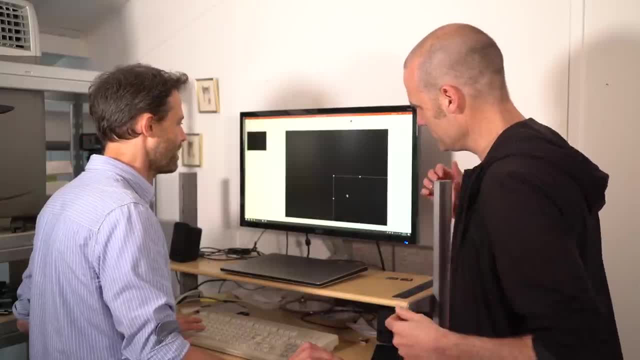 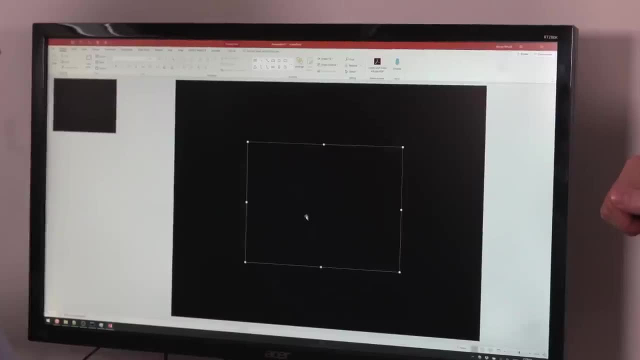 So we can't really see, but they're one and then the other right there, Yeah, Right, And then Actually we've got to do it one more time. Third one: Yeah, Slow down, Yeah, And that's going to go up here. 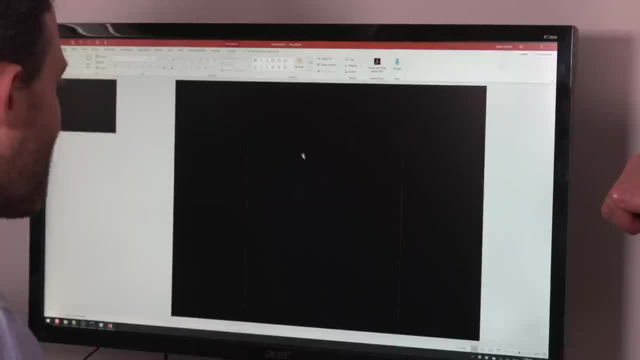 Oh, I like what's happening And it's going to go exactly in the middle, which is There? Okay, Now we're going to draw Insert. Let's see if you can guess where this is going: A giant triangle. 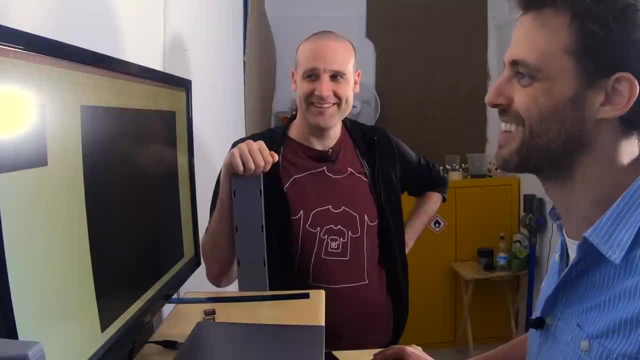 It better be a triangle And it's going to be the full width of the. It's just the size of the whole thing. Now, if I save this with the cryptic name T, let's say T. Now you can't see what's going on underneath. 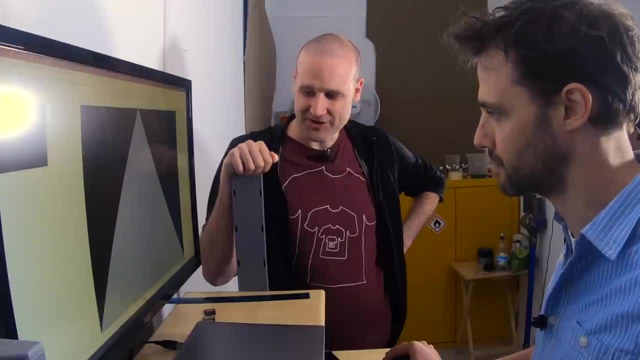 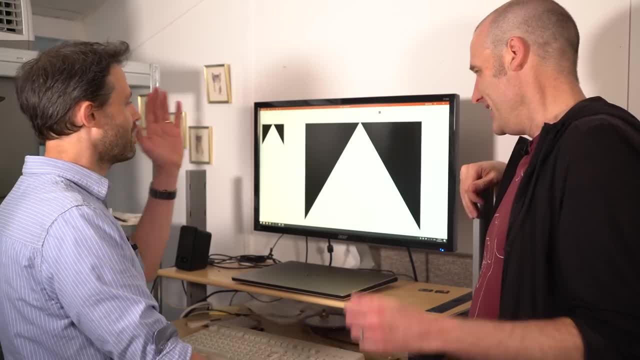 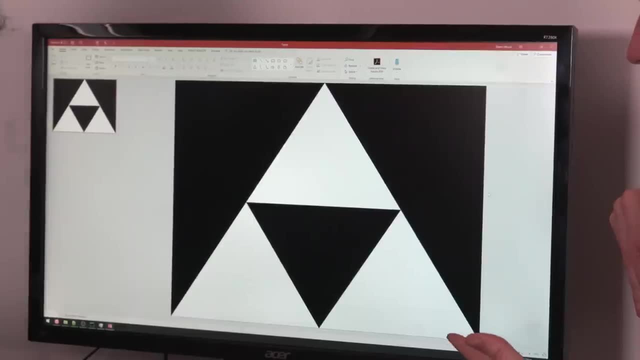 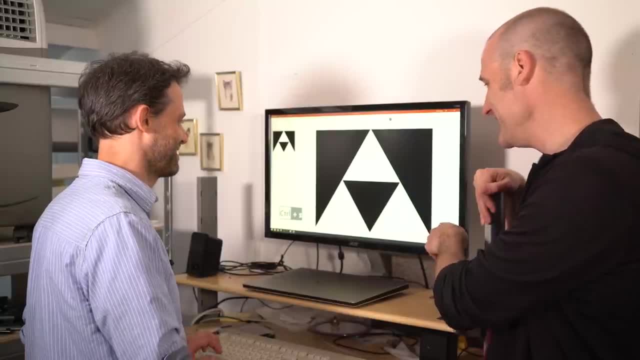 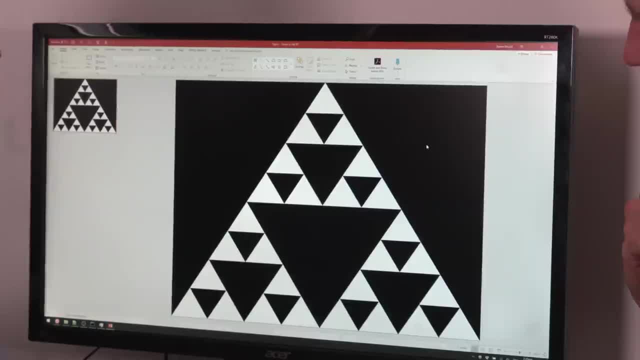 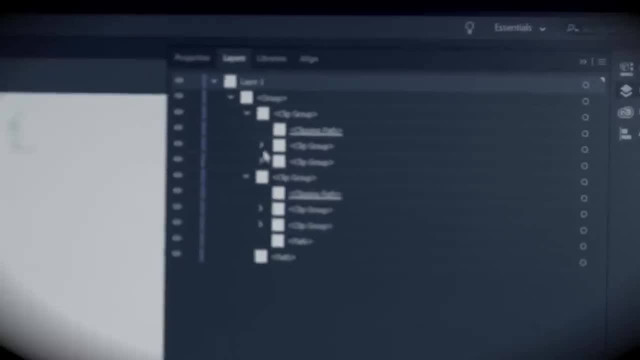 Yeah, And how many before it crashes. Okay, So let's see, Let's keep going. Is it taking longer each time? Each time it takes longer. And it's interesting because If you want to see Stephen and I pull apart the PPTX file and look at, 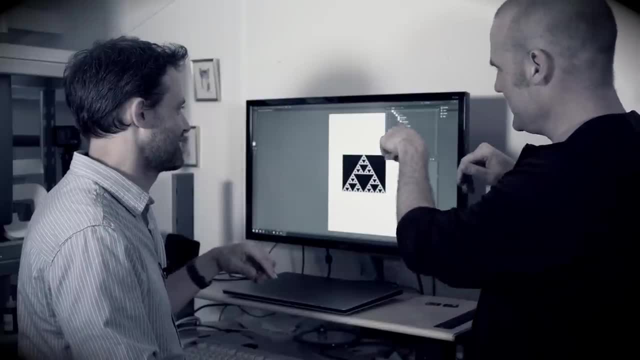 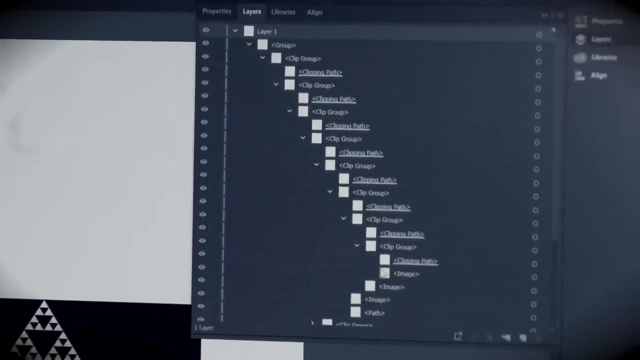 Exactly where the complexity is stored. that is in a separate video over on my second channel, along with all the details of exactly what version of powerpoint you need if you plan to try this yourself. for now, though, as soon as the final sapinski triangle is rendered, 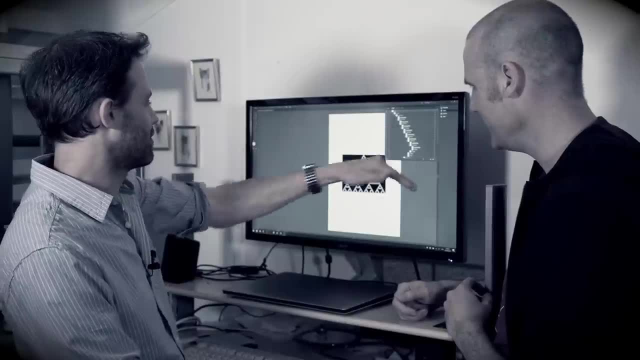 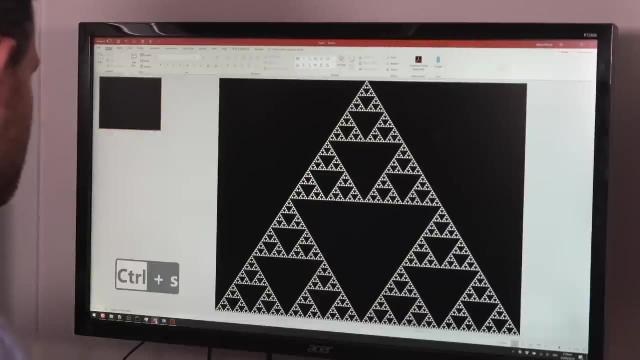 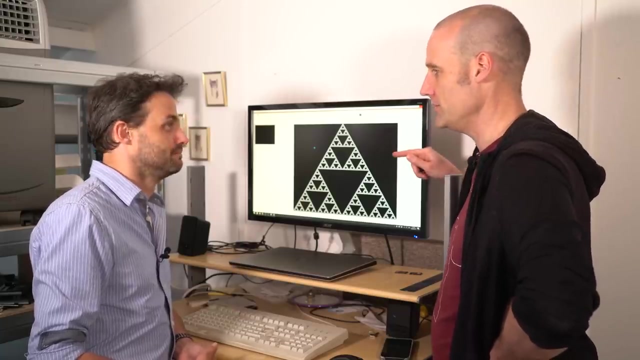 steve had one last amazing thing to show me. for steve's definition of amazing: one more, one more. you know what, while this is happening, we're going to take: we'll do the pose for the thumbnail of the video. yeah, good idea, is it? what is it? you're like i show you, you're showing me this and i should be. 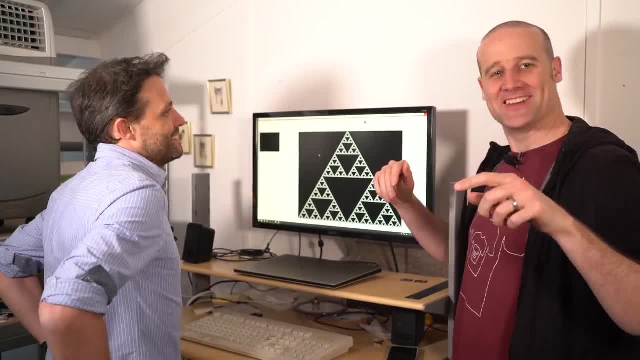 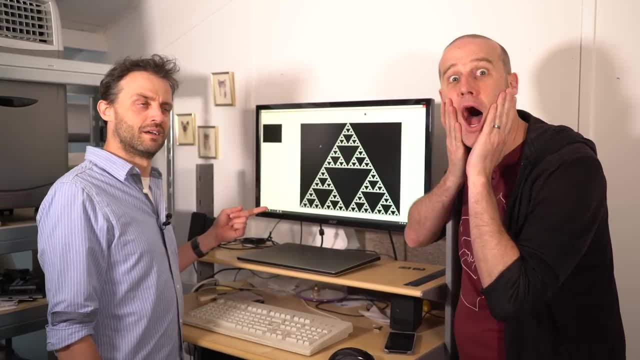 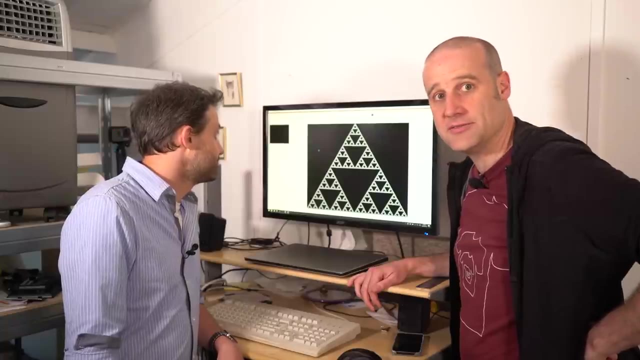 like, yes, i've got a reaction face to the this thing. yeah, i, i can, i can be like we're gonna get your face as well. what? if you're like looking at you know, like nailed it, that's the thumbnail. great, okay, you so? um steve, you have a youtube channel, don't you? i do there you are. it's called steve mold. 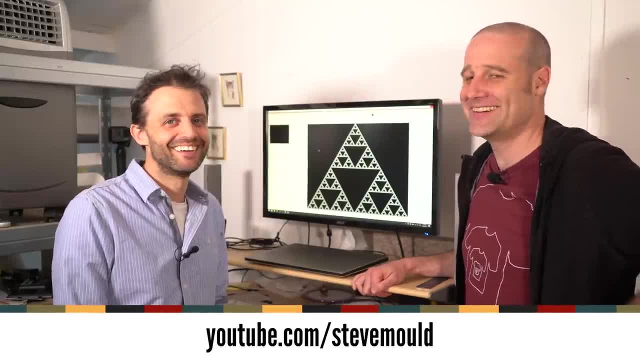 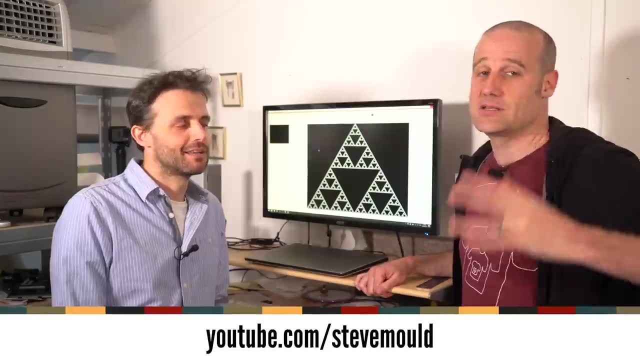 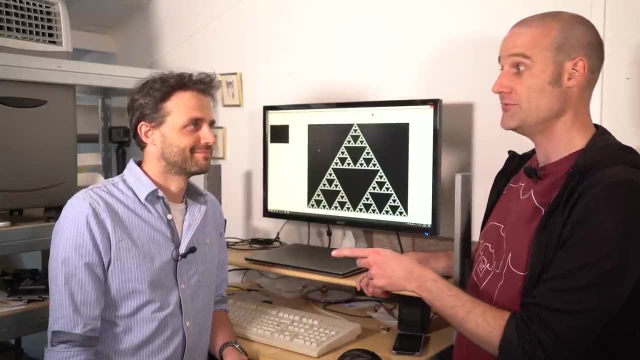 and it's steve mold's channel. yeah, yeah, i know, it's not so. steve does more physics than me, yeah, which is fine, and biology and chemistry- it's just applied things, yeah. so i do recommend you check out steve's channel if you don't already subscribe to that. and actually your most recent. 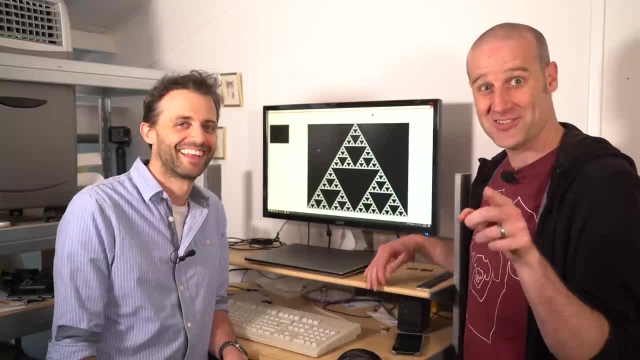 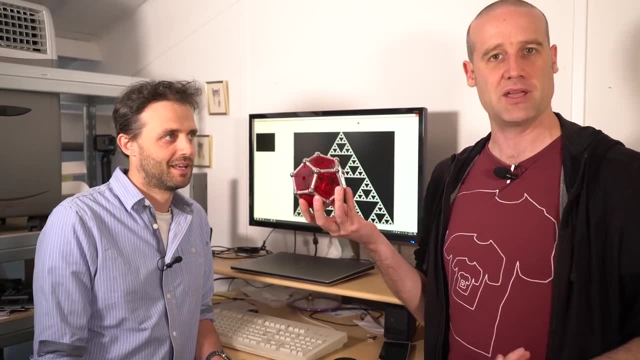 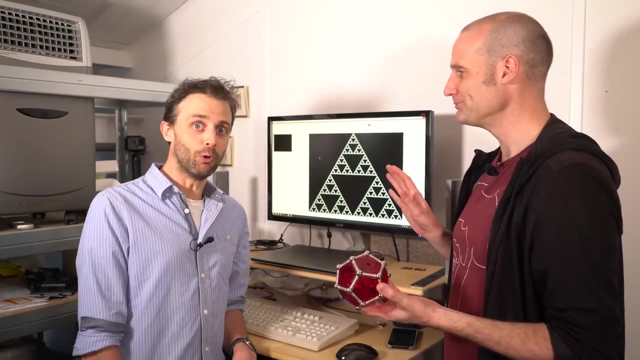 video at the time of recording is a good one, because actually it's over here and then you grab it. you did a thing with the dodeca hedron, yeah, so uh steve looked at how viruses uh replicate and assemble. so uh, so yeah, viruses are made of uh virus shells very often have icosahedral spoilers. oh so, so don't do it now. 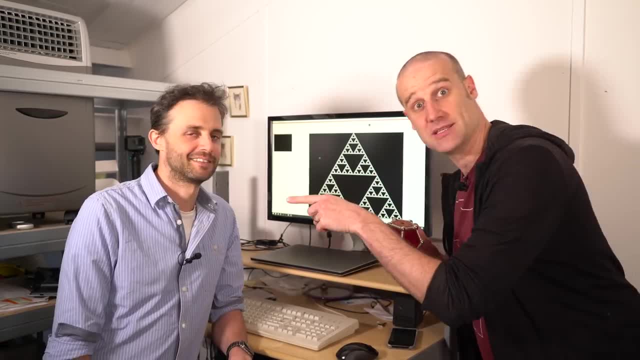 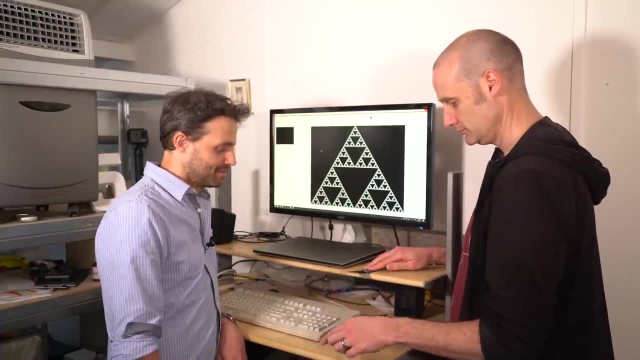 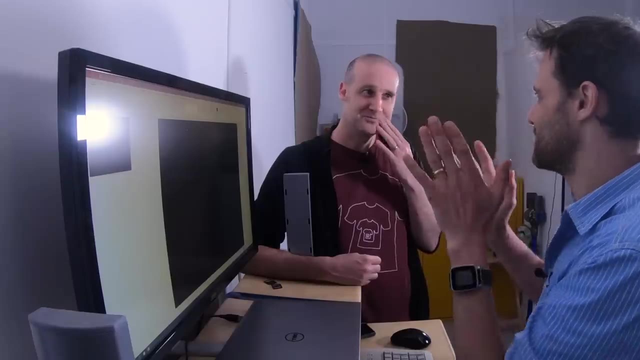 watch the video. i'll put a link below. it'll be at the end of this thing, so do check out steve's channel. yeah, yeah, we might have to give up on this one. okay, there's one last thing i want to show you. i wanted to figure out if i could do this right. 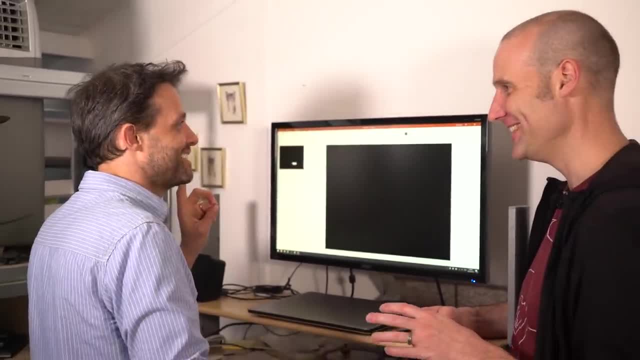 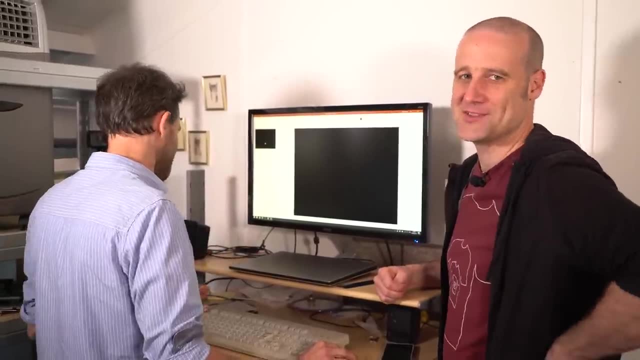 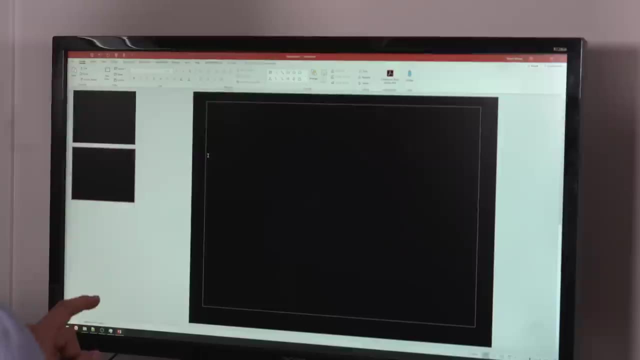 uh, and i worked it out, it's not a fractal. it's not a fractal, no, uh, it's a sequence. see if you can guess. there we go okay, recursive sequence. you say steve, okay, so we've got, we're gonna have actually two slides, right, right, um, this second slide is like a holding slide for. 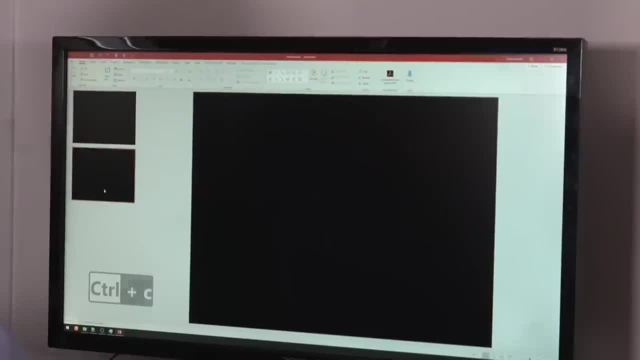 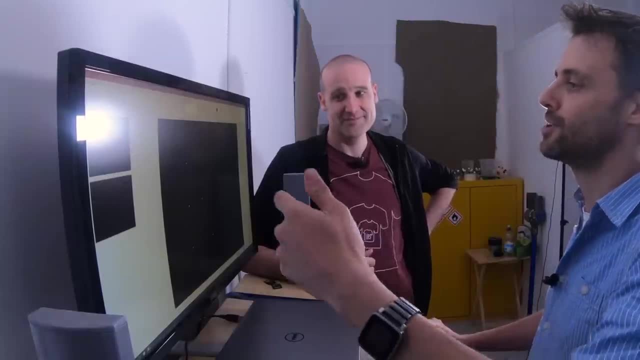 the first one. so i'm going to take and copy the first slide- yeah, copy that. and then i'm going to copy that and then put a copy of that into the second second slide, which is just storing it. so, yeah, it's storing like. so this is going to be like one step behind, if you, if you see what i mean. 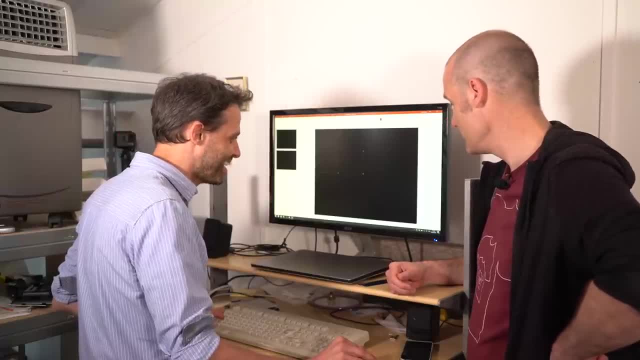 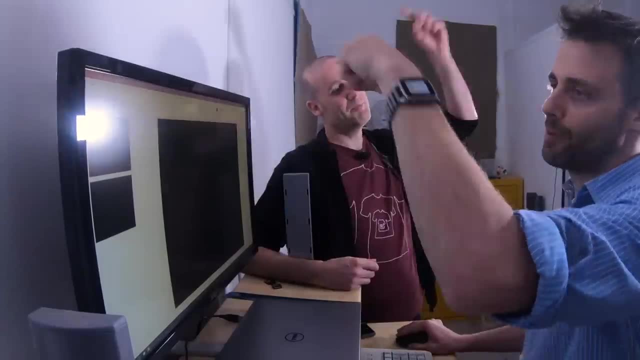 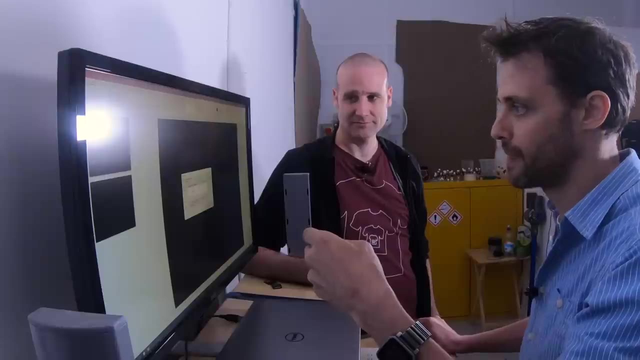 i think i know exactly where you're going. okay, um, i mean, in a way, it's two steps behind, because actually this, this one, has one behind and two behind, right, right. so so the first slide is going to have a copy of itself and the next slide 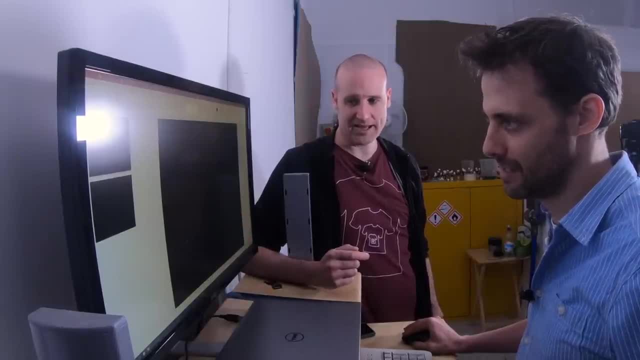 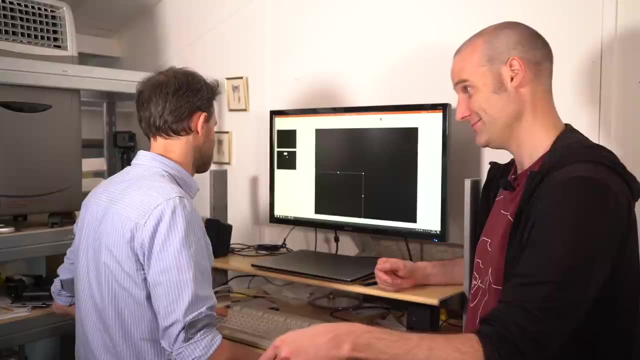 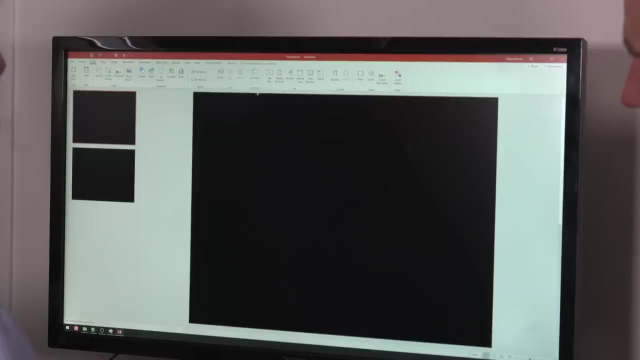 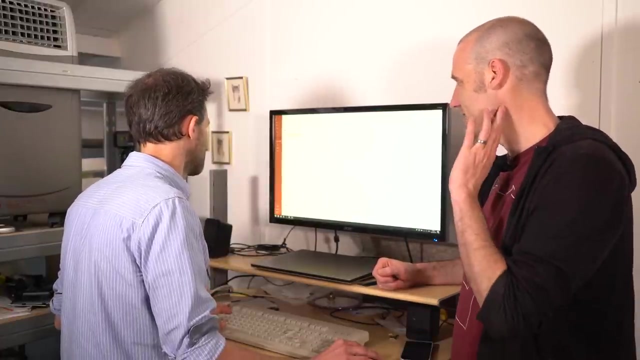 right, so it's going to have a copy of itself and it's going to have a copy of the second slide, which is a copy of what the first slide was, the slide before, yes, and then we're going to put a white square in the top, uh, like. so right now we save. oh, we haven't saved it. there's anything there?